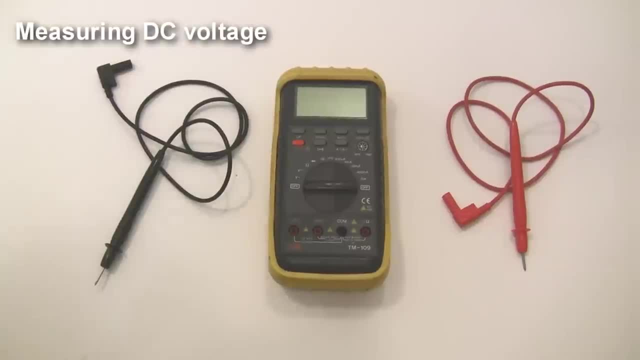 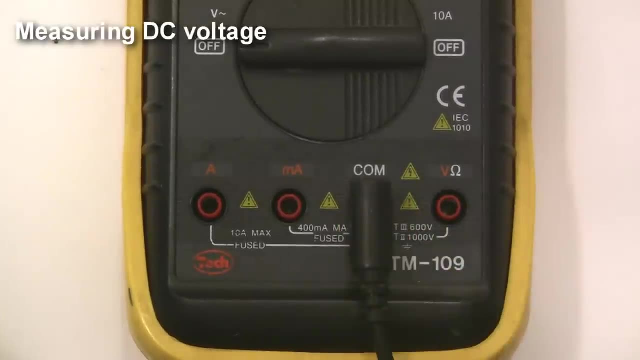 Okay, so now you have a multimeter. how do you use it? Let's start with measuring DC voltages. First, check the cables, Make sure the black lead is in the jack labeled COM or COMMON, And once it's in there, you'll never need to take it out, because the black lead always goes to COMMON. 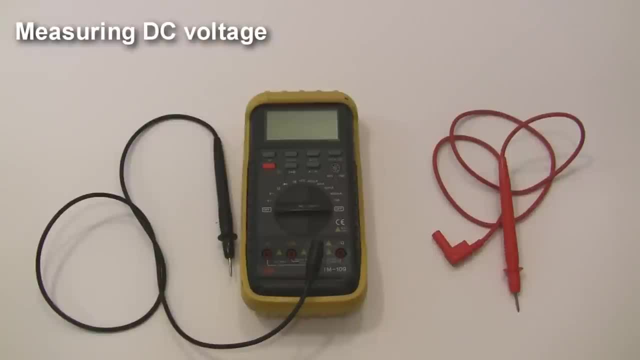 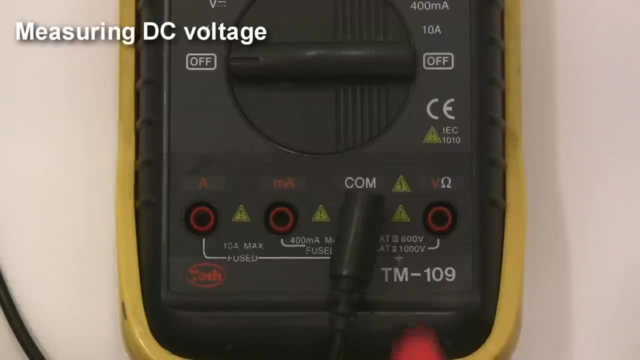 The red probe, on the other hand, is something you'll have to pay very close attention to. If you plug it into the wrong jack, you will blow a fuse in your multimeter. We want to measure voltage right now, so I'm plugging in the red lead into the jack labeled VOLT. 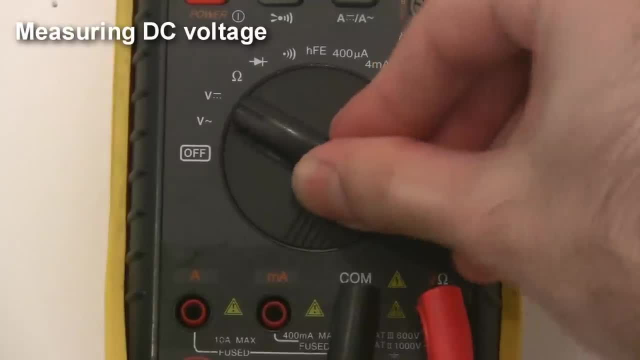 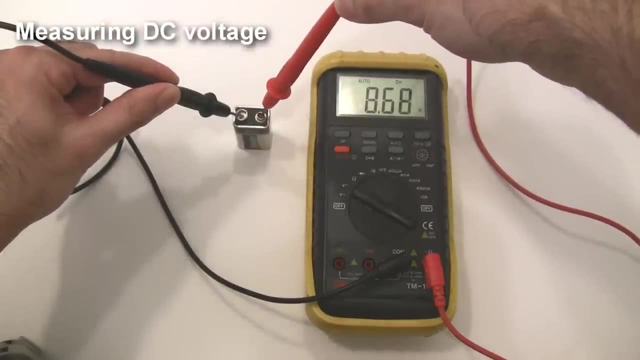 not amps. Next, set the dial to measure DC voltage Touch the red probe to the positive terminal of your device and the black probe to the negative terminal of your device, and you should get a voltage reading. If you get the wires backwards, that's okay, you'll just get a negative reading on your multimeter. 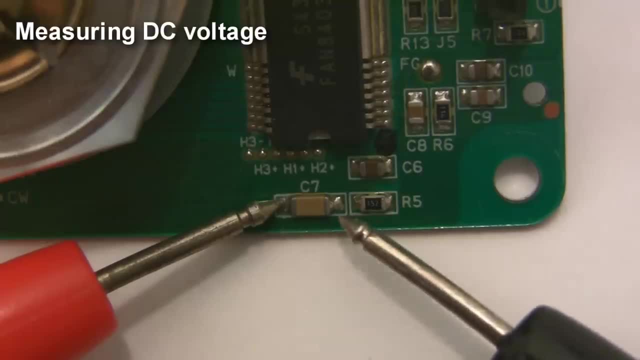 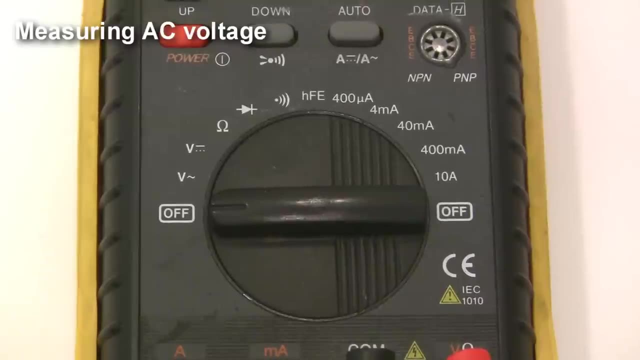 And that's actually a good way to figure out polarity. Now you can measure voltages in pretty much any DC circuit, as long as you're careful to not short anything out with the metal probes. Okay, let's move on to measuring AC voltages. 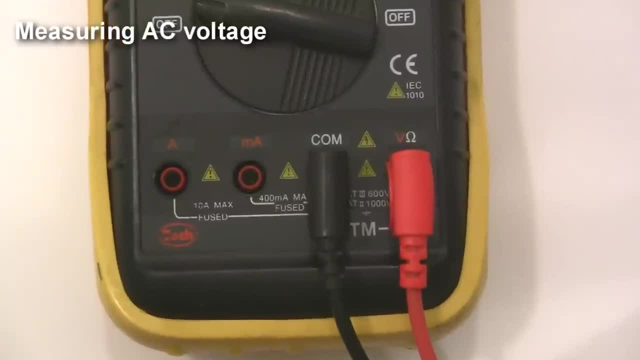 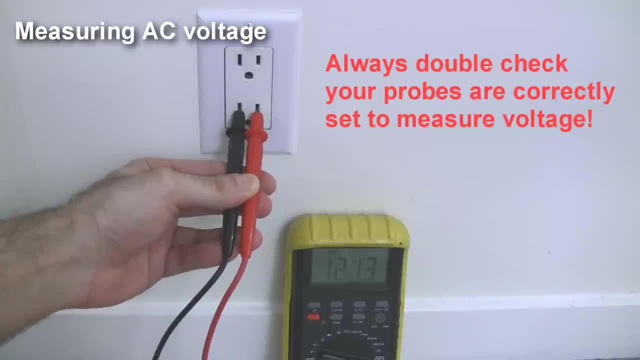 Set the dial to the AC voltage setting and again make sure the red lead is in the jack labeled voltage. Touch the probes to the AC voltage source that you want to measure and you'll get your reading. As long as you don't touch the metal parts of the probe or short them out, this is perfectly safe. 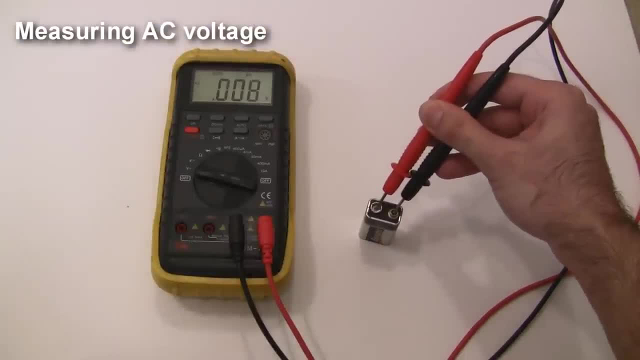 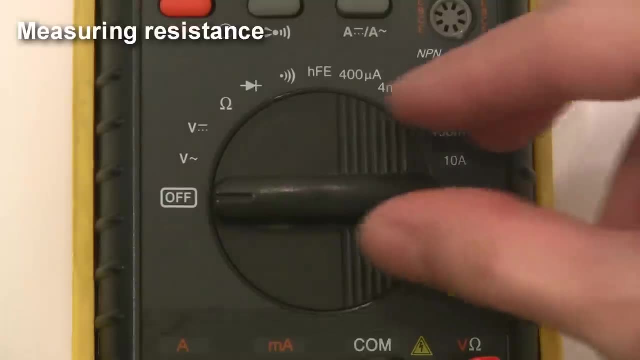 And, as you would expect, there's no AC voltage coming out of this DC battery. Measuring resistance is easy too. Make sure the red lead is in the jack labeled ohms for resistance and set the dial to the resistance setting. 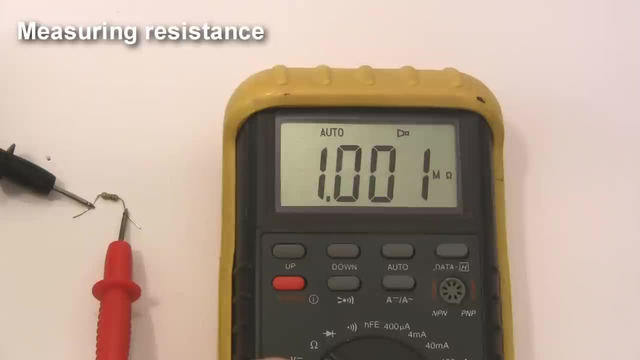 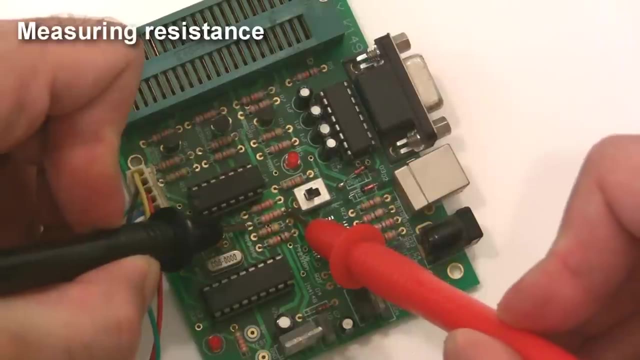 Here is me measuring the resistance of the skin on my hand. Here is me measuring the resistance of a resistor, And here I am measuring the resistance of a speaker. Now you might be wondering if you can measure the resistance of something in a circuit. 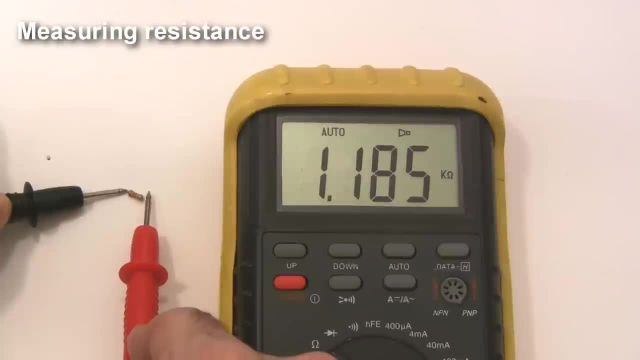 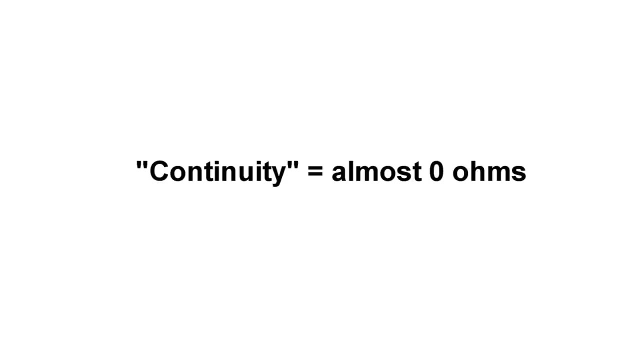 Well, unfortunately it most likely won't work. You're going to have to remove the resistor from the circuit before measuring it. Next, let's talk about continuity. Measuring continuity basically just means checking whether or not there's a good connection between any two points in a circuit. 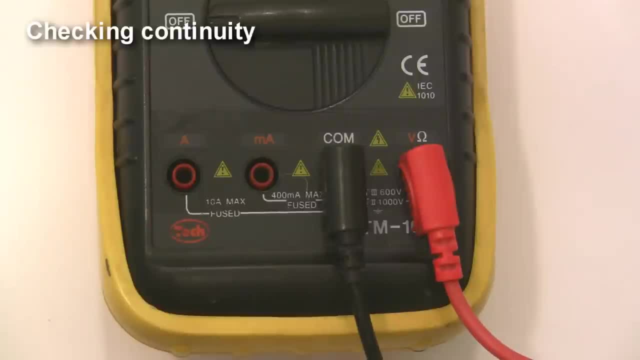 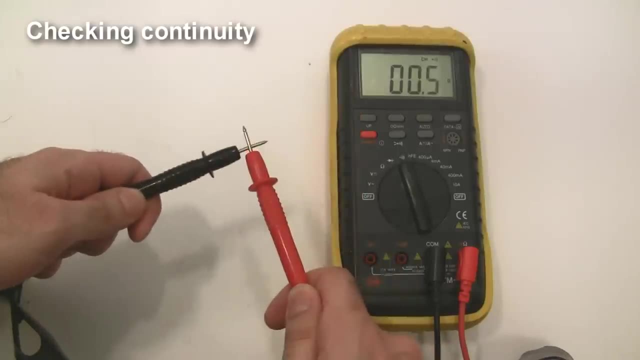 To measure continuity. make sure your red probe is in the jack labeled continuity, or in my case resistance, and set the dial to the continuity setting. Test that the continuity function is working correctly by touching the probes together. Whenever there's almost zero resistance between two points, the multimeter will beep.